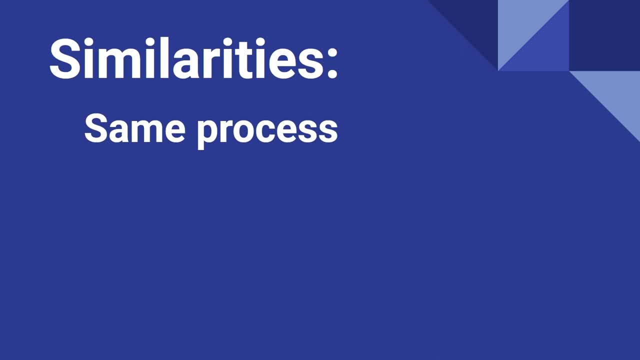 in this field. you probably don't need to know their finer details For information purposes. there is a client and server handshake process, followed by a key exchange, followed by the encryption of data sent between client and server. For the client and server handshake process, 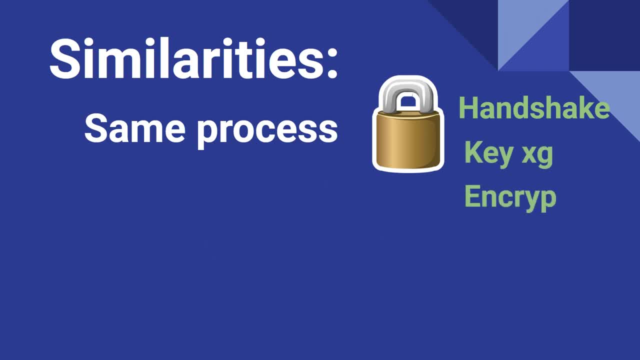 there is a key exchange, followed by the encryption of data sent between client and server. For the client and server handshake process, there is a key exchange followed by the encryption of data sent between client and server. If you'd like a little more information on how that process works, we have a separate video that 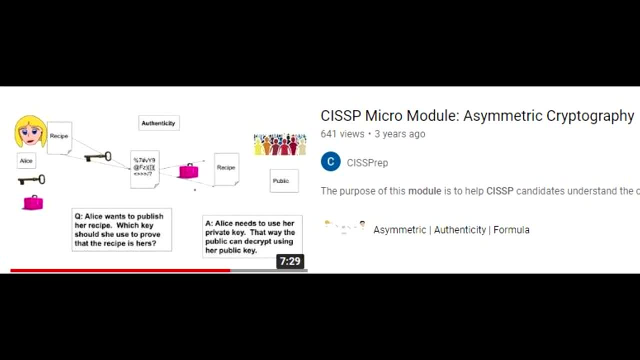 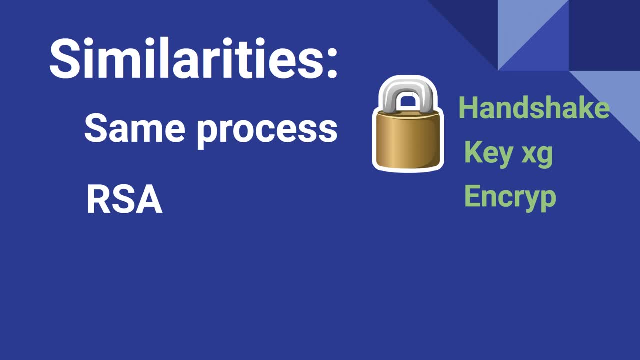 covers asymmetric encryption, so I recommend watching that, where we explain with visuals how the process works. Both protocols can use an algorithm called RSA or Rivest Shamir Adelman for key exchange, And the terms SSL and TLS certificate mean the same thing, In other words. 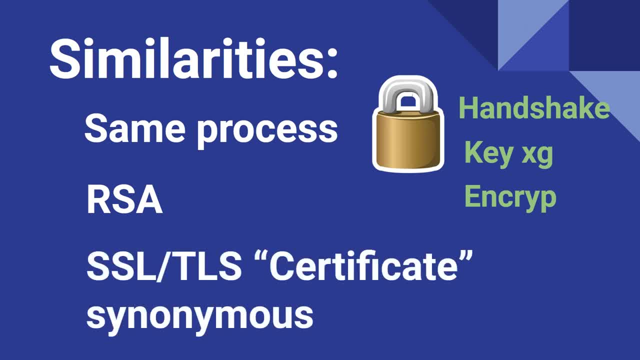 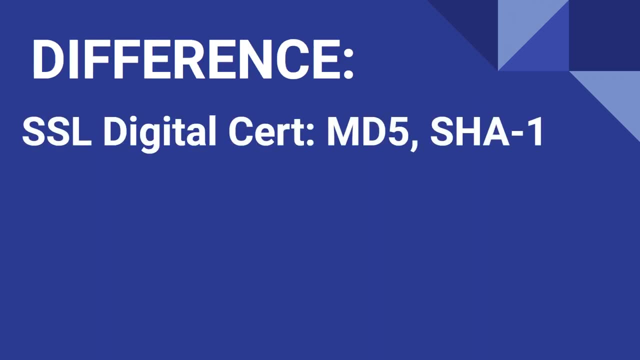 if you say to someone that you have a TLS certificate or an SSL certificate, it basically means the same thing. These terms are often used interchangeably in the industry, So now let's look at some differences. One of the main differences can be the use of hashing functions. SSL can use older hashing. 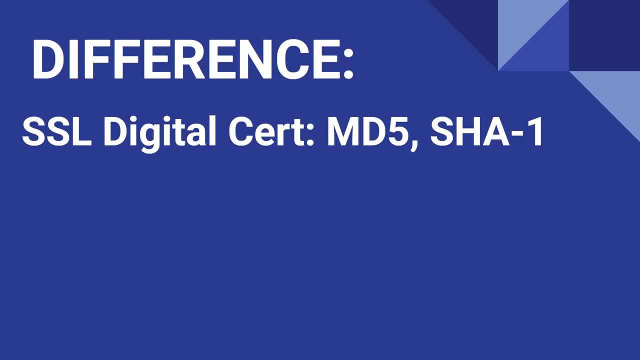 functions such as MD5 or SHA1, which have been shown to be deprecated due to the ability to produce something called a collision. A collision is when the digest or digital representation is shown to be the same when there are different inputs. If you'd like more information on hashing, 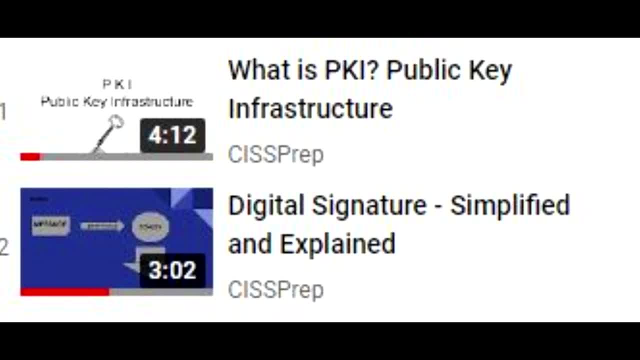 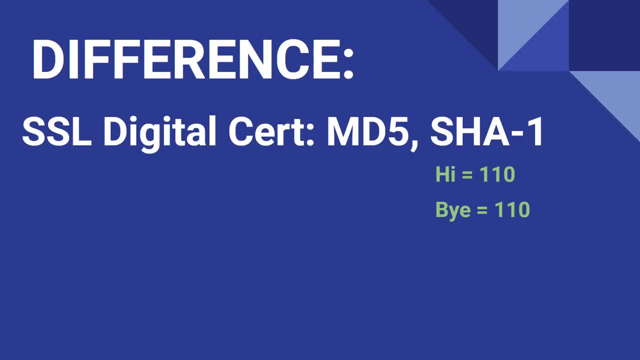 functions. we have a few videos on hashing digital signatures or digital certificates. that covers this information, with some nice visuals too. Ideally, hashing functions should never produce the same output, given any change to the input. TLS uses SHA256,, which is called 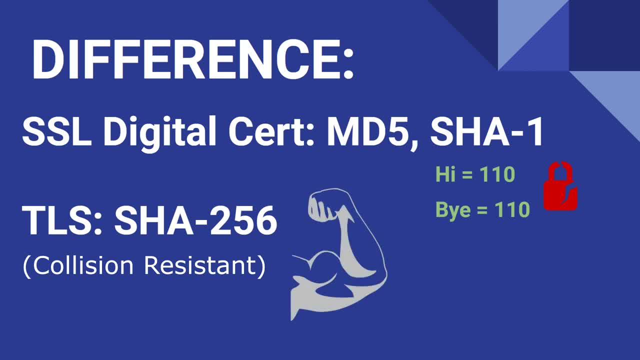 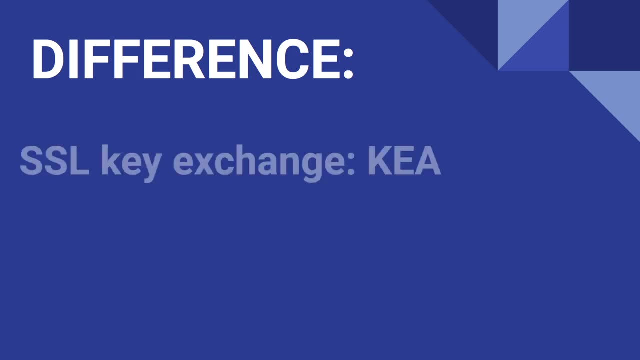 collision resistance. In other words, you can have an infinite number of inputs that will never produce the same output, at least with today's modern computing power. There are also some differences in the algorithms used for key exchange. We previously mentioned that both SSL and TLS can use RSA. SSL can also use 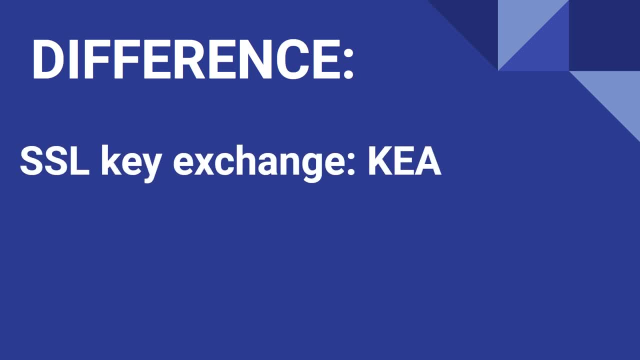 KEA, or key exchange algorithm, which is based on Diffie-Hellman. TLS uses Diffie-Hellman or DH variations, which are asymmetric algorithms, or PSK, which stands for pre-shared key protocol. Once the handshake process is complete and a symmetric key is agreed on, SSL uses the data.